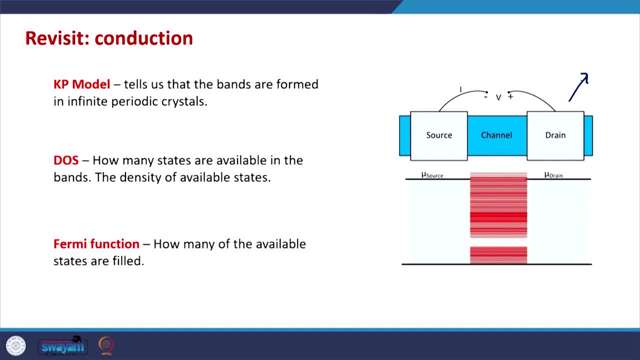 device that we are trying to understand. we are trying to understand the mechanism of conduction or transport in a 2 terminal device And a 2 terminal device generally. this middle region, the channel region, is taken to be a very small region. the source and 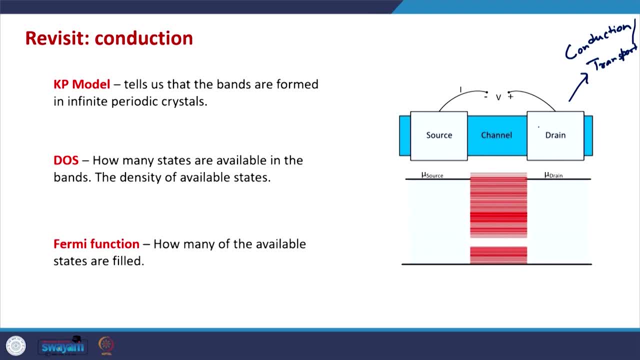 drain regions which are essentially like metal, Yes, Meta metal or moving metal, 처럼 In the metal here, the emitting should be say 1 Ya, and it must have a low pressure ột each thing. datum of Grid: delta square. if that is the case, then you had already 1 Ya, and 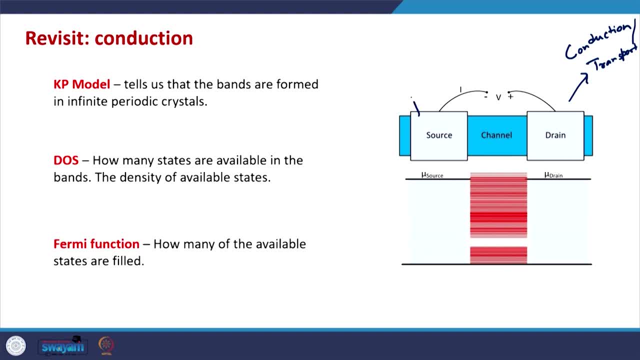 metals or which are like metallic contacts. these are much bigger than the channel region. So the channel region is, in a way, a mesoscopic system and the source and drains are microscopic and that is why we need to understand the density of states in the channel region in 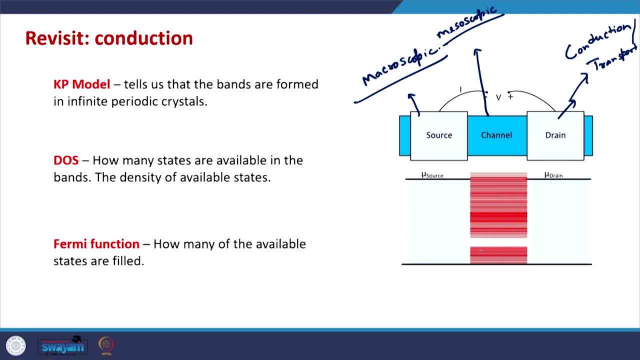 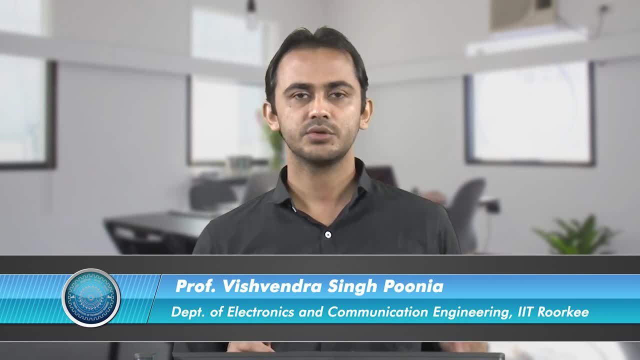 order to see how many allowed electronic states are available at a given energy, and we saw that the conduction depends on the available electronic states between the source Fermi level and the drain Fermi level when we apply a voltage. that is what we saw in the last. 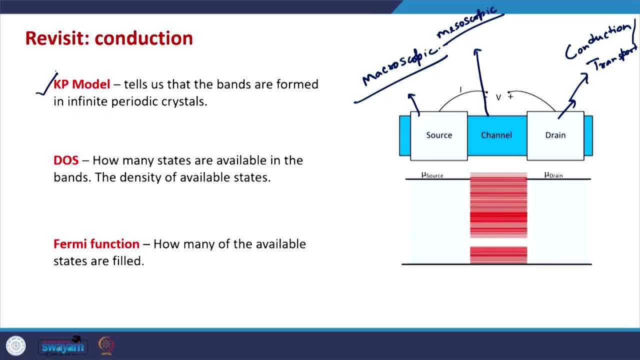 class. So we have gone through the Kp model, which tells us that in infinite periodic crystals bands are natural, Naturally formed. we have also understood the idea of density of states, which basically tells us how many allowed electronic states are available as a function of energy. how? 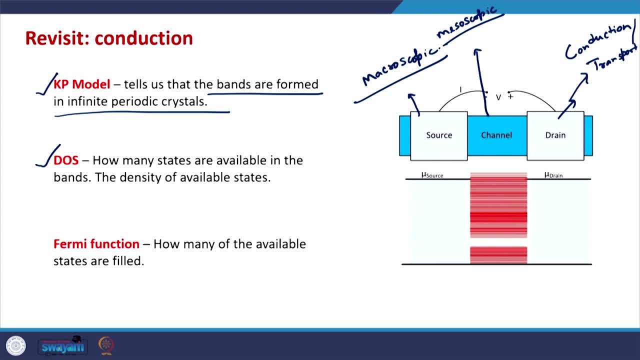 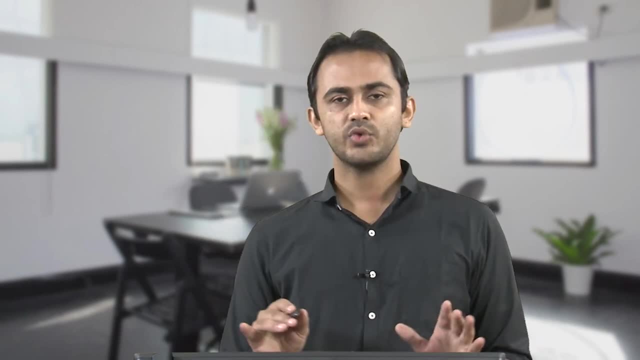 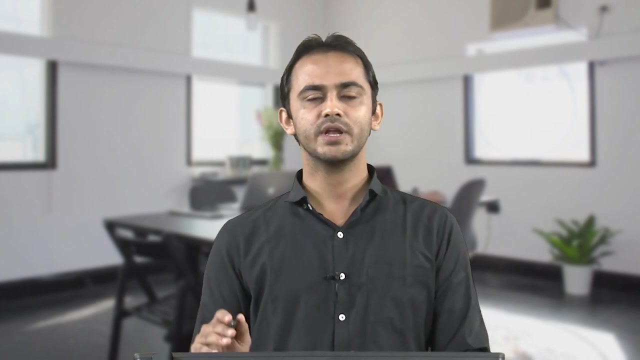 many allowed electronic states per unit volume, per unit energy. Now, finally, what we need to see is how many of the available electronic states are filled with the electrons in equilibrium. So when there is no transport, No transport, there is nothing happening in the device in equilibrium situation. how many? 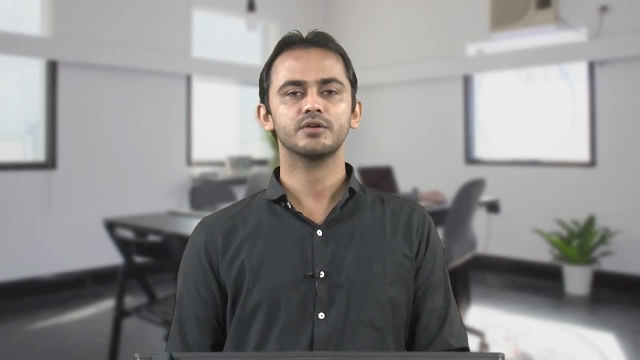 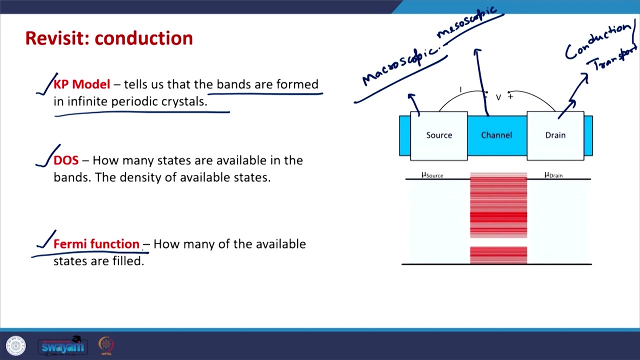 of the available electronic states are filled and how many of them are empty, And that is governed by this function, which is known as the Fermi function or Fermi Dirac distribution function. This comes from quantum statistics and one of the main concepts that play an important 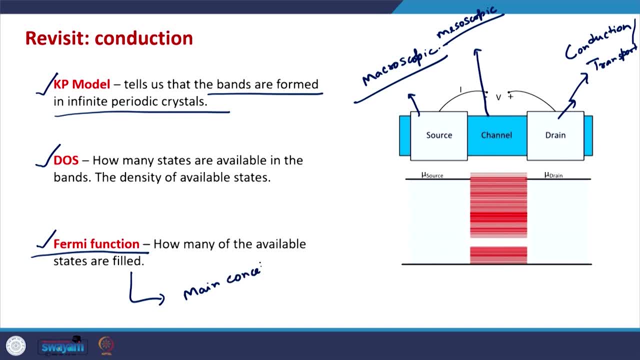 role. role here is the Pauli's exclusion principle. So please keep in mind this is, this, is this. distribution is an equilibrium concept. So there are two kind of. generally we talk about equilibrium and we talk about steady state. sometimes we also talk about the transient. 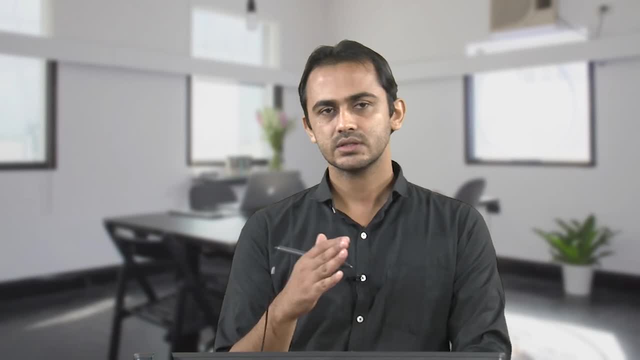 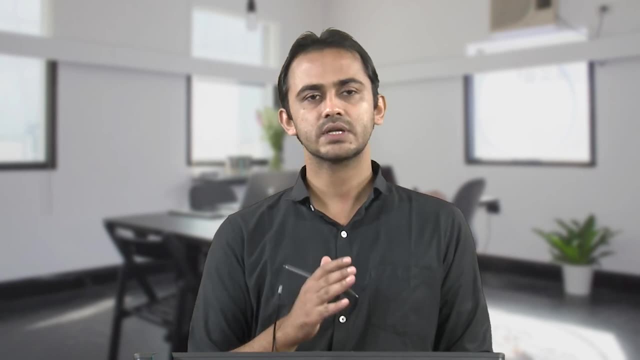 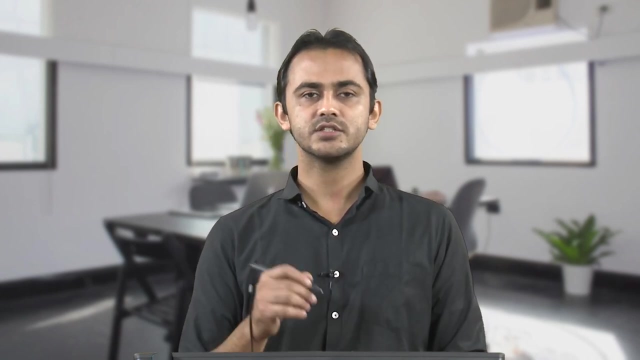 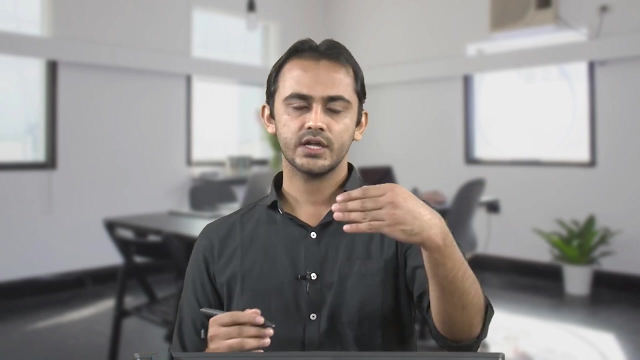 states actually. So there is. there is important difference between these three situations in equilibrium, as I told you in previous one of the previous classes, that each and every process in the system is countered by the reverse process, is balanced by the reverse process. So if energy or if number of particles are flowing in one direction in equilibrium, 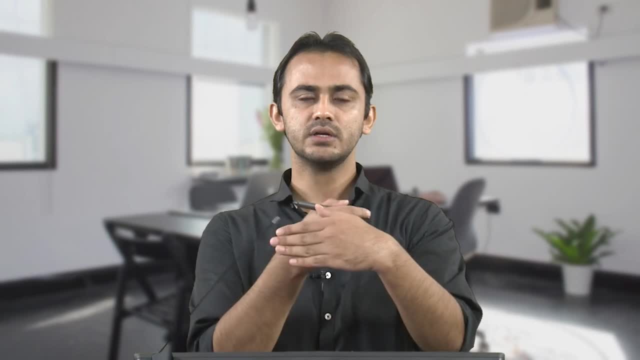 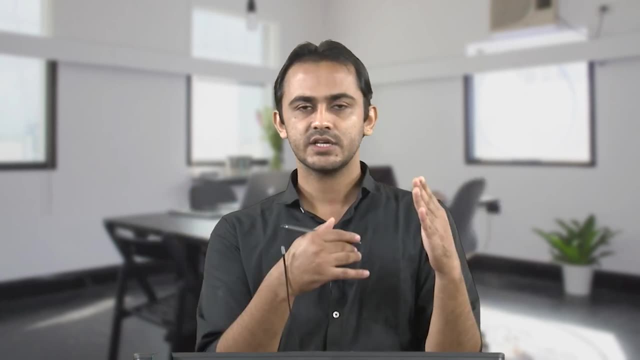 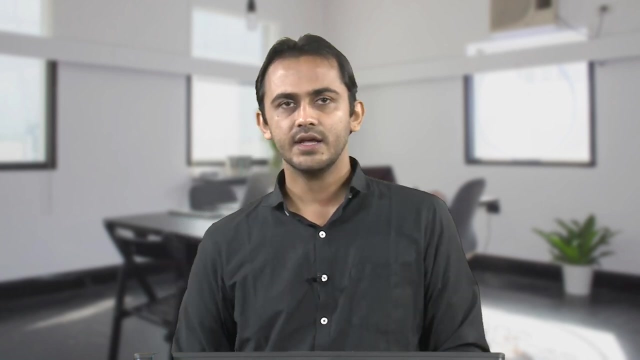 the equal amount of energy or number of particles will be flowing in the reverse process, So that ultimately, each process is balanced by the counter process. So, resultantly, nothing is happening in the system. Second idea is the idea of steady states. in steady state the system is So in steady. 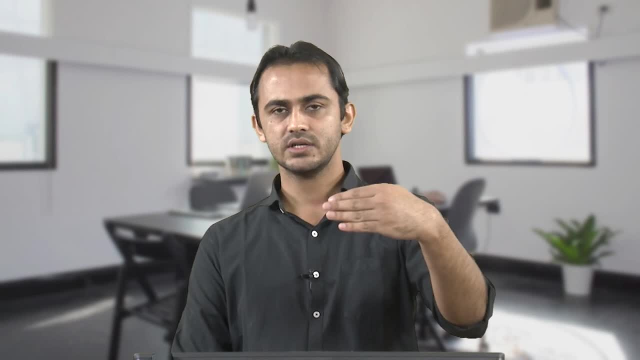 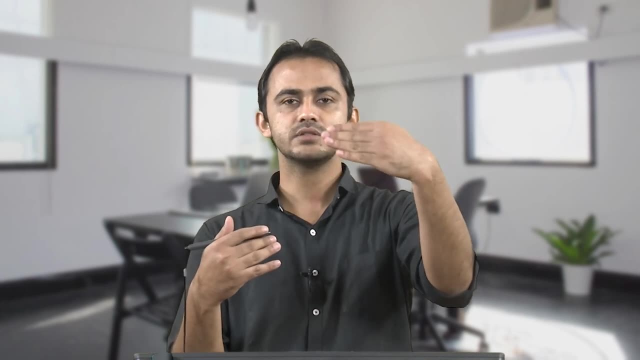 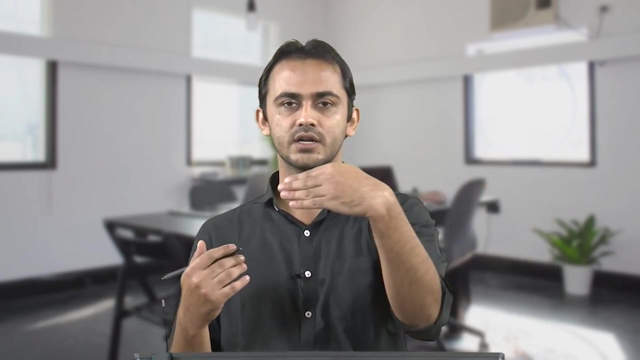 state a process is happening in one direction as compared to the other direction. So this is happening. So the rate of change of variables is 0.. So, for example, if n number of particles are flowing from left to right in a device and n by 2 number of particles are flowing, 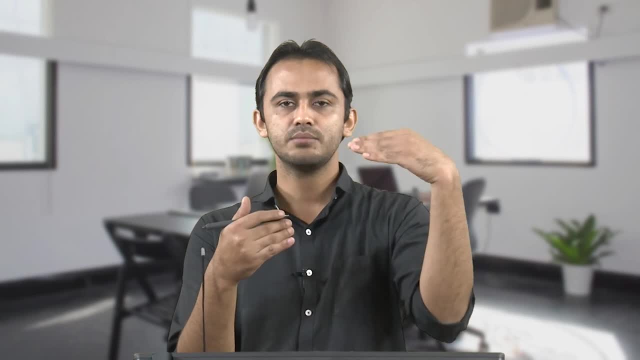 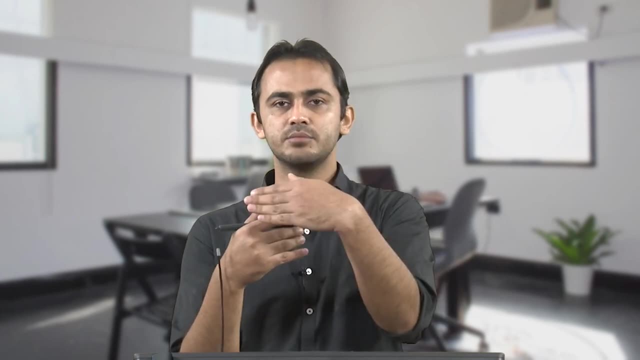 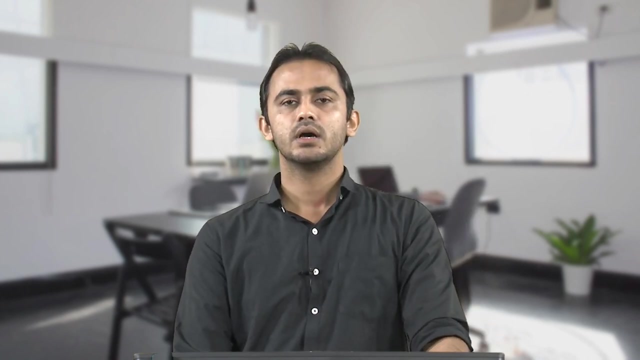 from right to left in a device. So resultantly, n by 2, number of particles will be flowing from left to right. So this number of this resultant number, this net number of particles, will not change with time. So that is the idea of the steady state In steady state. 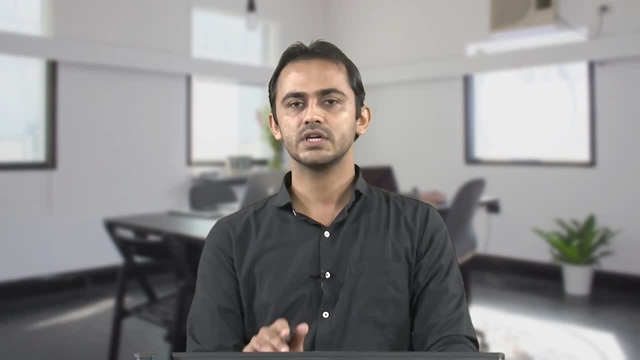 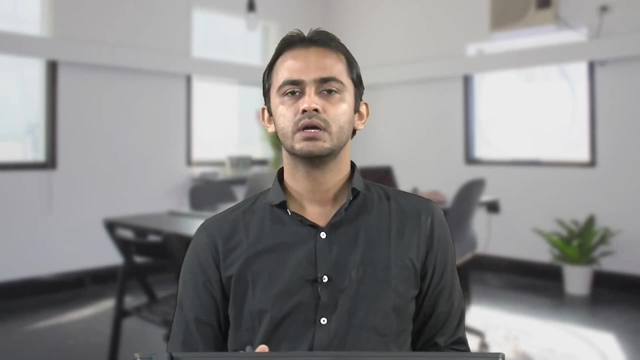 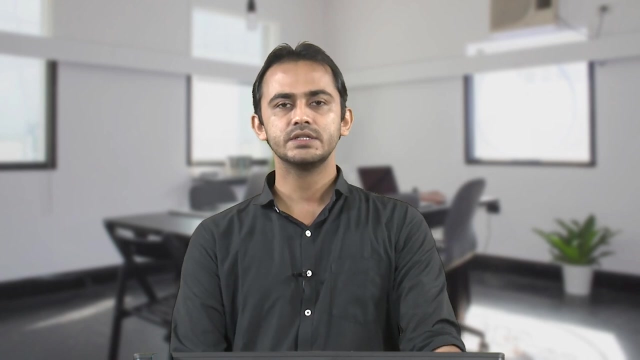 there is a net flow of energy particles or there is a net, I would say, a process happening in the system, But that process is constant with time. that is not changing with time. So generally our device analysis is done in steady state generally when we do ihv characteristics. 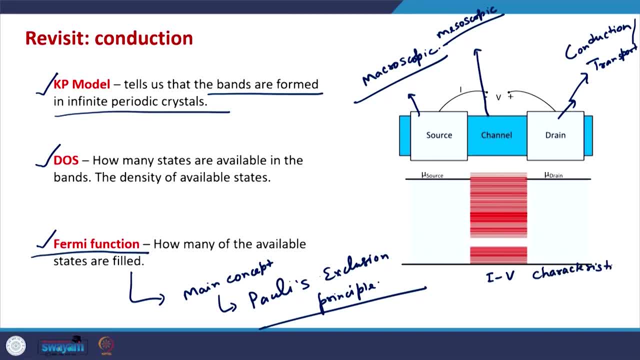 calculations generally. we assume steady state. we assume steady state Sot hat electron, that electrons are flowing from one direction to other direction, but this flow is constant. 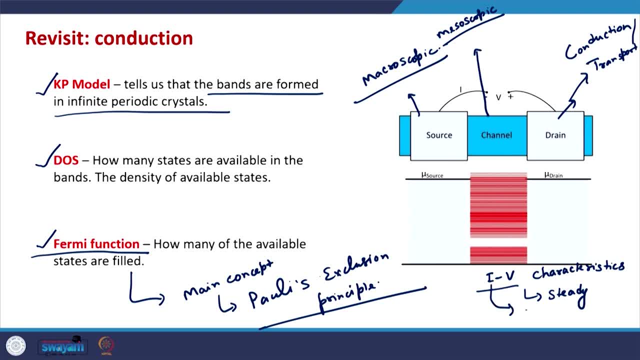 This is not changing with time, which means the current is constant at an instant, Although we can change the voltage, which will change the current, but it will very soon come to the steady state and that is where we do the analysis. When we suddenly change the voltage in a device, it will suddenly change the current, and that 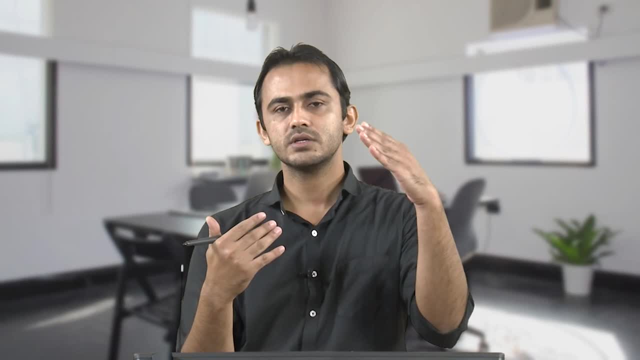 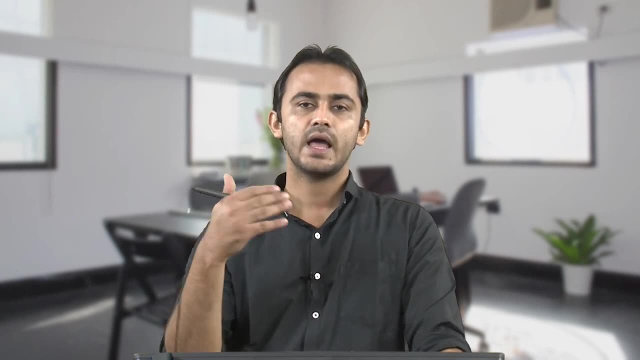 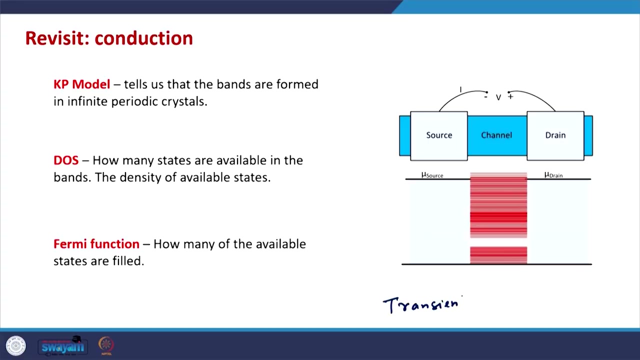 is the moment when this rate of change of current or this current will not be constant. It will be changing with time and that is known as the transient state, when the system variables are changing with time. So that is the transient state of the system generally happens when we suddenly change. 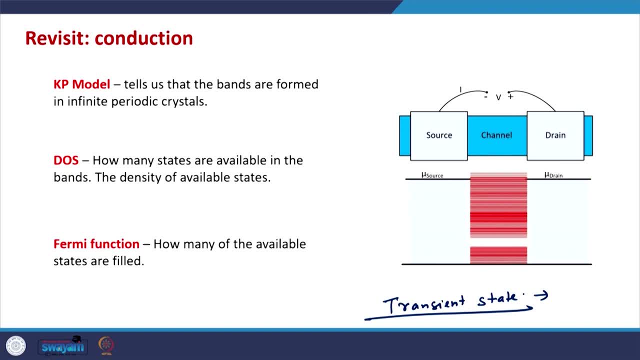 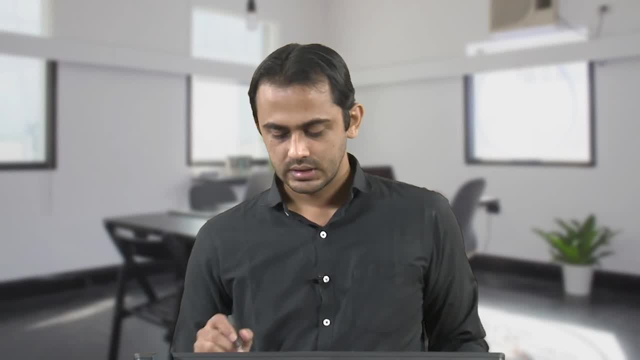 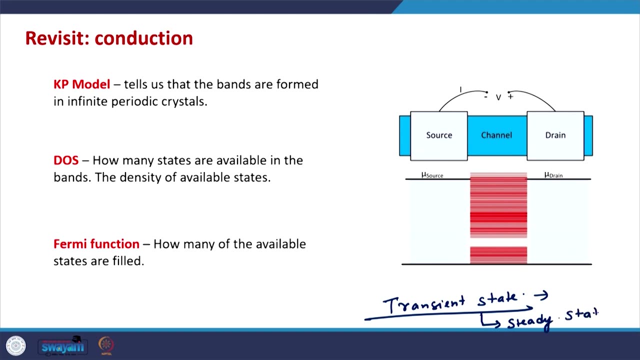 the force Or suddenly change the action in the system, suddenly change the voltage applied on a system. Generally, most of the system, most of the stable systems. they quickly go to steady state. They quickly attain a steady state, specially in our solid state devices. although this analysis 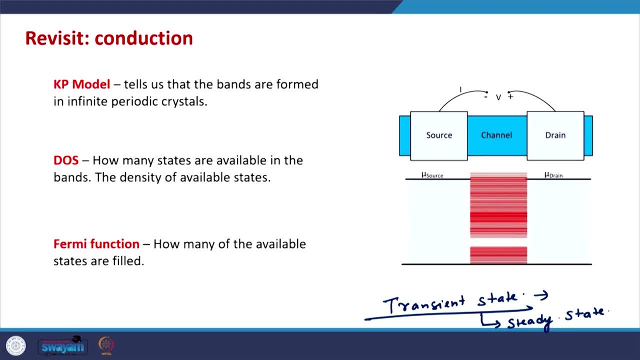 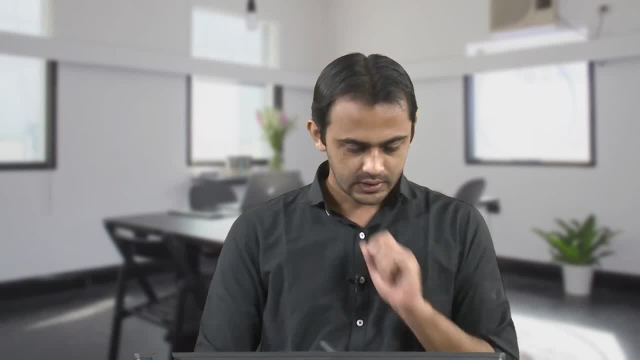 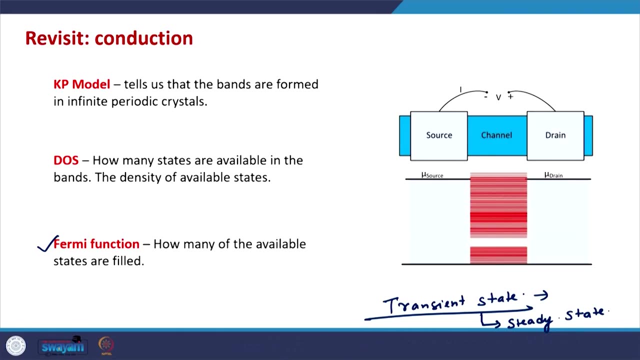 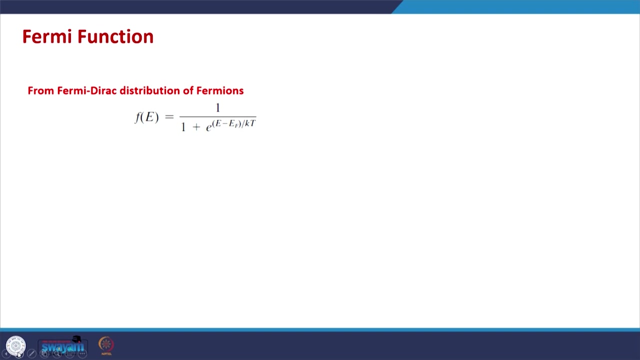 is in detail done in control theory and control systems, which is sort of out of scope of this course. So now we will see how Fermi function, or Fermi Dirac distribution function, governs the distribution of electrons in various energy states, in the solids or in the in any system. 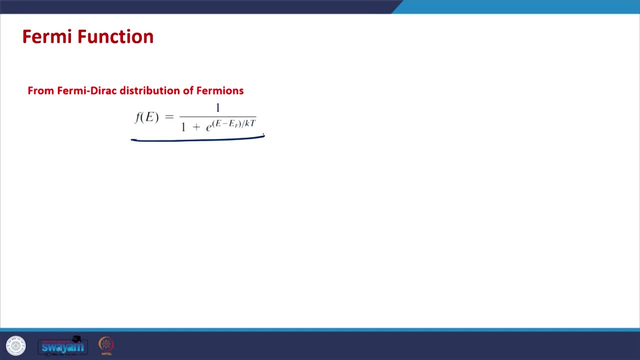 So this is essentially the Fermi Dirac distribution function. We discussed in last class that fundamental particles can generally be categorized in two categories: One is fermions, Second is bosons. Second is neutrons. Third is neutrons. Fourth is neutrons. 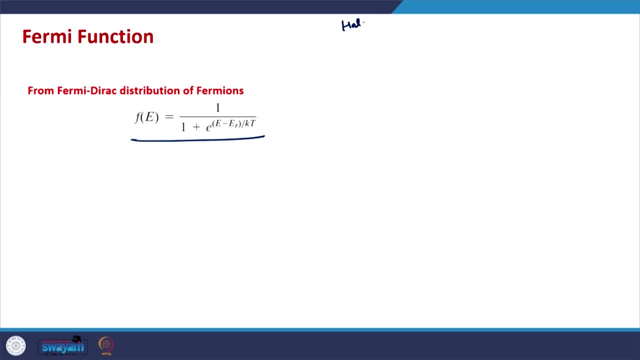 Fermions have half integer spins. So fermions have half integer spin and bosons have integer spin, including spin 0. So they follow. these are the fermions. Fermions follow Pauli's exclusion principle. So what Pauli's exclusion principle says is that no two fermions can occupy the same. 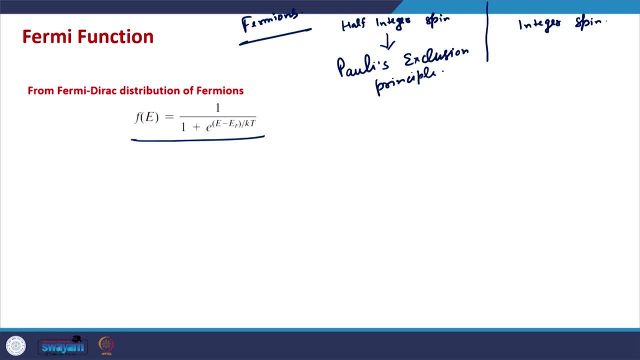 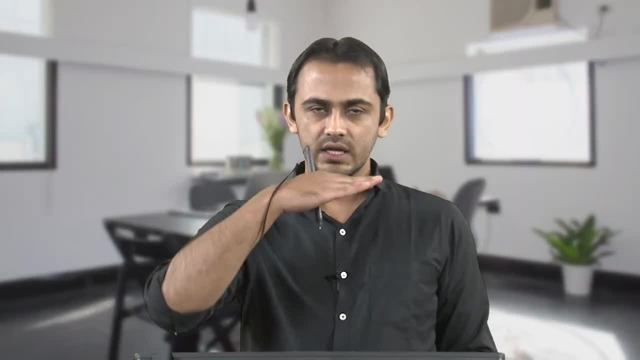 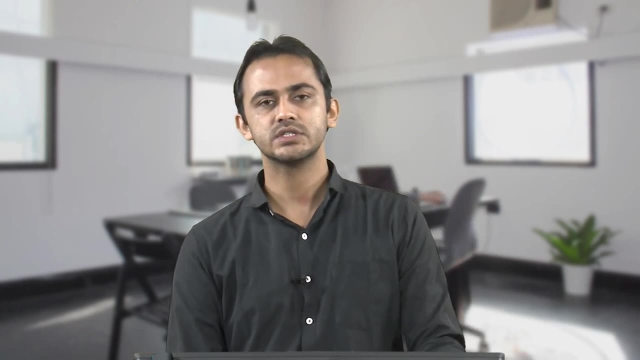 quantum state. They, no two fermions can have the same set of quantum numbers. What it means is that a single electronic state, single electronic level, can only occupy two electrons of opposite spins, So that all the quantum numbers are not same for the electrons. 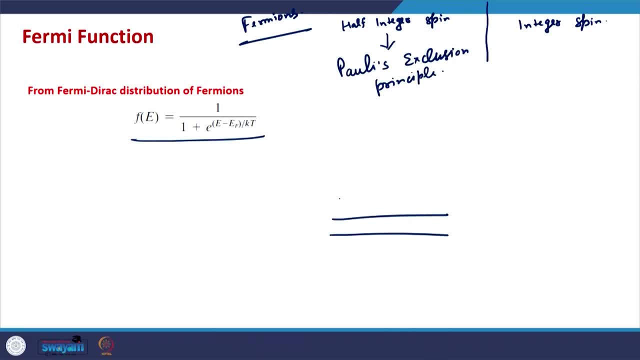 So if we have, for example, In a system, if we have these kind of energy levels, discrete energy levels, each of these can take two electrons of opposite spin. Each of these level cannot hold two electrons of the same spin because that is not allowed by Pauli's exclusion principle. 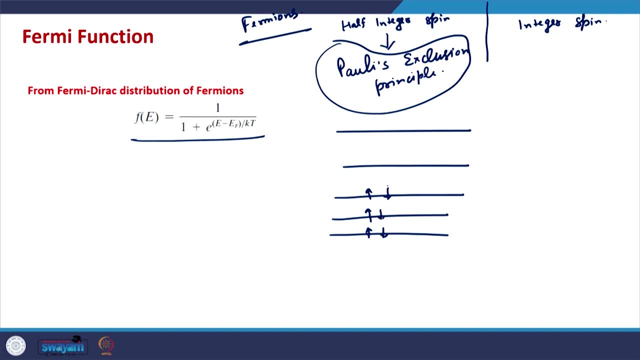 Similarly, this level can also hold, and this level can also hold- two electrons of opposite spin. However, in bosons, if these are the discrete energy levels, many particles can exist in single electronic state. There can be many, many particles in the single electronic state, generally at room temperature. 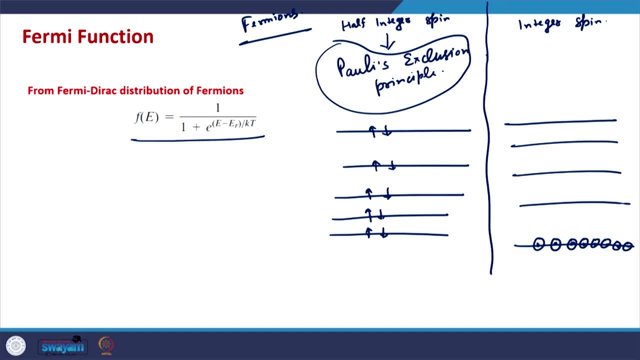 some of these particles are in higher energy states, So the distribution of electrons. 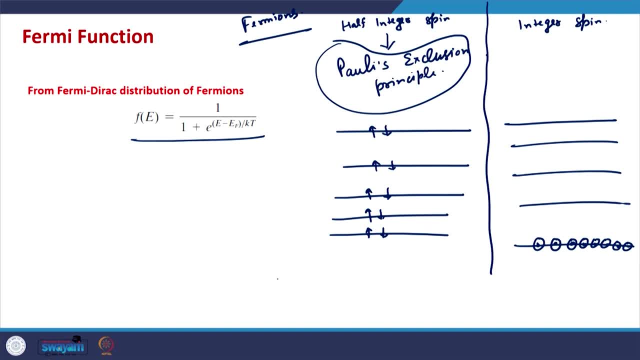 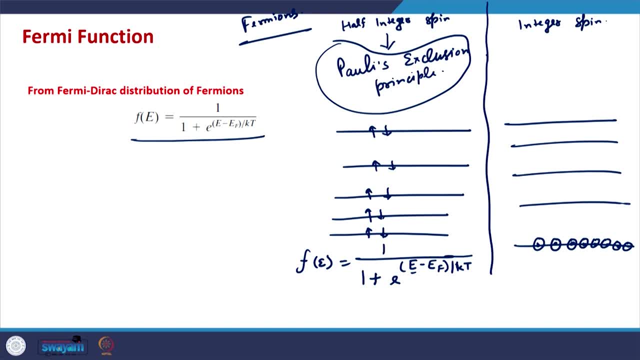 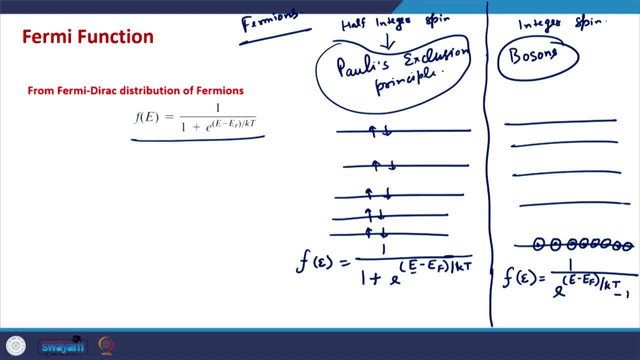 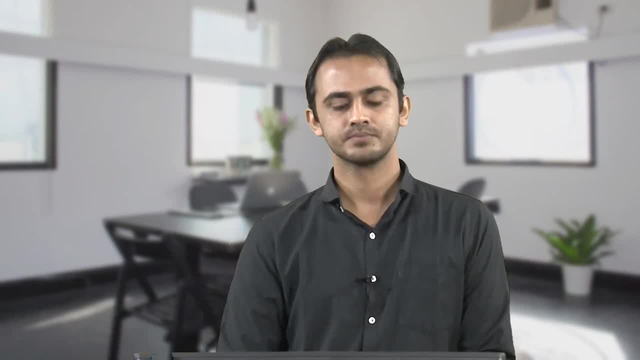 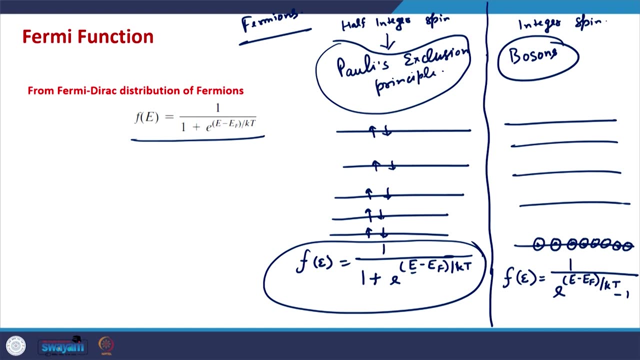 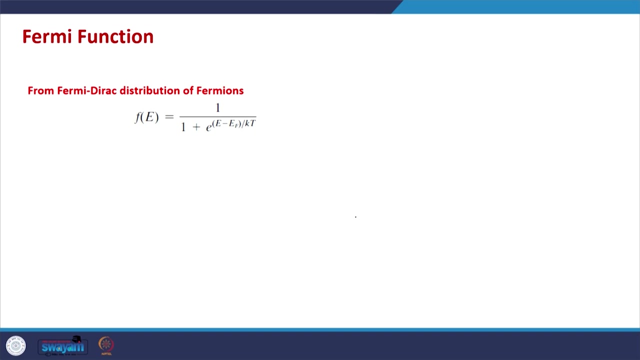 So this is the probability with which an energy state will be occupied by the electrons at a given temperature. So there is, there is another way of understanding this. let us say we have a system. There is actually this probabilistic argument of Fermi Dirac. distribution function needs to be understood properly Because 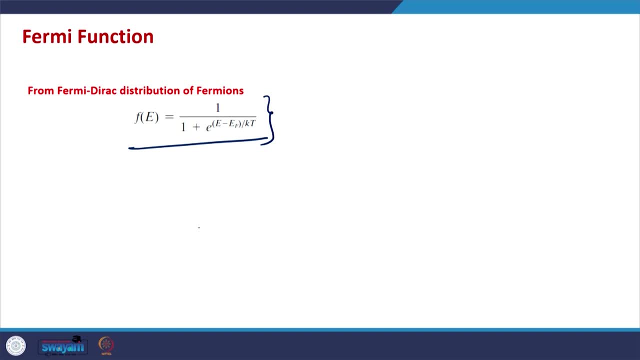 need to see where this probabilistic interpretation basically arises from. So if we have a system in which there are various energy levels, let us say there are six energy levels and let us say the energy of each level is 1 eV- the energy of the ground- 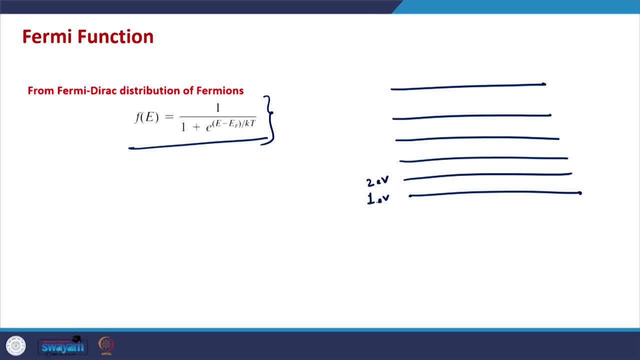 energy level. the lowermost energy level is 1 electron volt. the second energy levels energy is 2 electron volt, third one is at 3 electron volt, fourth one is at 4 electron volt and fifth one 5 and sixth one 6 eV. Generally, this is not how energy levels are distributed. 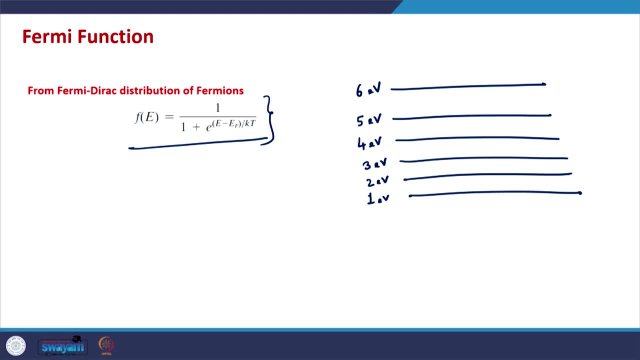 in solids generally, the distance between energy levels increases gradually as we go up in actual atoms. But this is just to understand how electrons will be distributed in a system. So now, if we have 8 electrons in this system, then at T equal to 0 temperature, let us say: 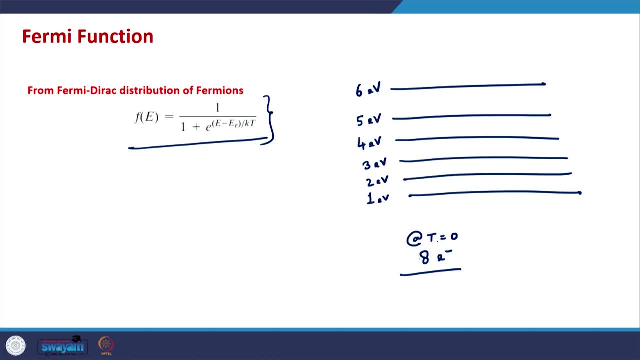 we have 8 electrons in this system at T equal to 0 temperature, when all the electrons are in their ground states, so to say they do not have any thermal energy, all the electrons will be at the lower possible, lowermost possible energy state. 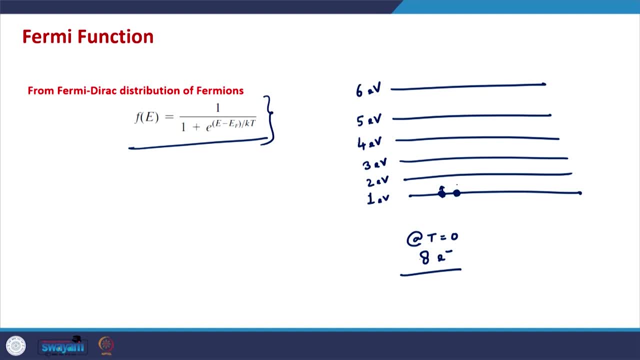 So two of these electrons will occupy the ground state, one eV state. two of these electrons will occupy the 2 eV state. similarly, 2 will occupy 3 eV and 2 electrons will occupy 4 eV state. 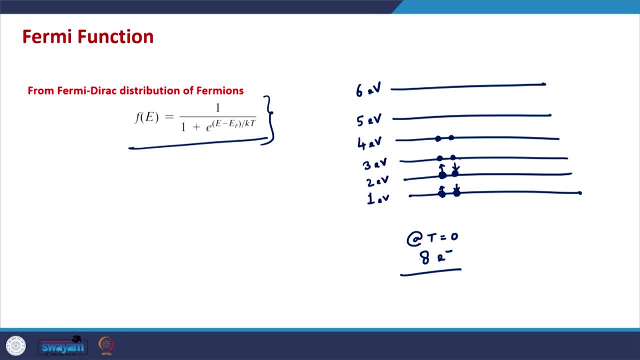 So that is how electrons will be distributed in the in various energy levels: in the solid, at T equal to 0 Kelvin, when there is no thermal energy in the system and all the electrons are sitting in their lower most energy configurations. And for these two energy levels I have also shown the spin levels, so that the Pauli's 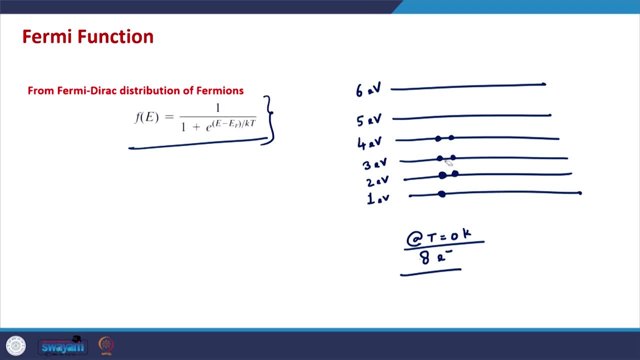 equation principle is not violated, but let me remove the spin level from these electrons. So this is how electrons will be distributed at T equal to 0 Kelvin. But now let us say that we are at room temperature, at, or let us say at, 300 Kelvin temperature. 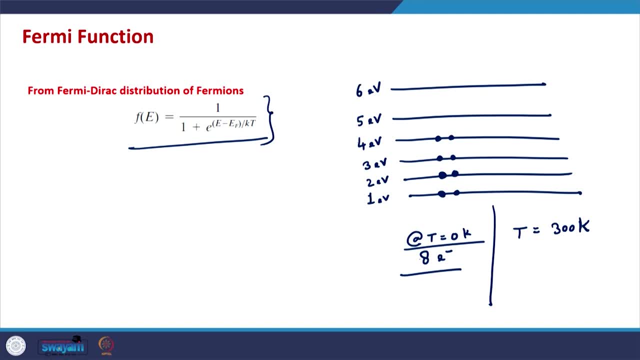 So at 300 Kelvin temperature, electrons will have some thermal energy as well. they might, ah, They will be having this additional amount of k? T energy coming from the thermal energy, and let us say ah. So at T equal to 0 Kelvin, what is the total energy of electrons? 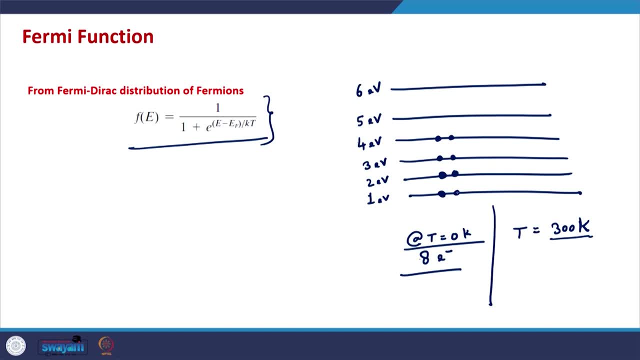 So 1 electron, 1 e v for this, 1 for this, 2 e v, 2 for this, 2 for this, 4 e v, 3, 3, 6, 4, 4, 8.. So 8 e v here, 6 e v here, 4 e v here and 2 e v here. 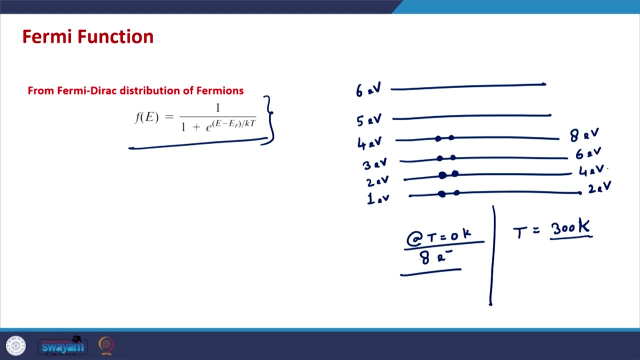 So in total, electrons will have 20 e v of energy at T equal to 0 Kelvin. ok, Now, at room temperature, let us say the energy of electrons now is, let us say, 30 e v. just for an example, just, it is not the exact figure. 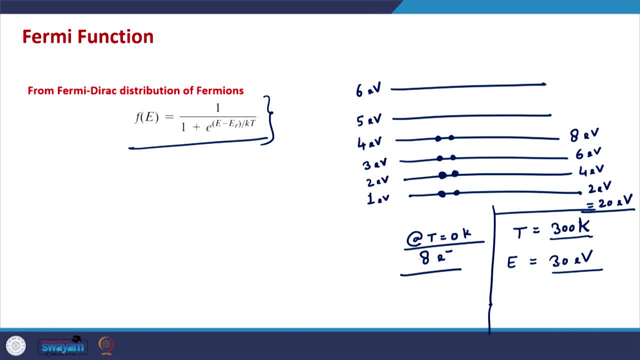 Just at a certain temperature. let us say the energy is increased by 30 e v. TI is equal to 0 Kelvin, So the size of the room temperature of time I have 1,, 3 over 0. So time D is of 30 now and 3 over 0. 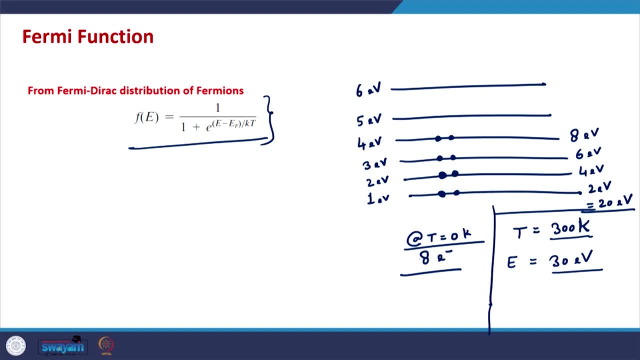 So in total, E v of T will equal to 0 Kelvin. Okay, And as room temperature, let us say the energy, 30 eV. So now what can happen is so, with 30 eV energy, how many electronic configurations are possible? So one of the possible configurations is that: so if 2 electrons are here, 2 are here. 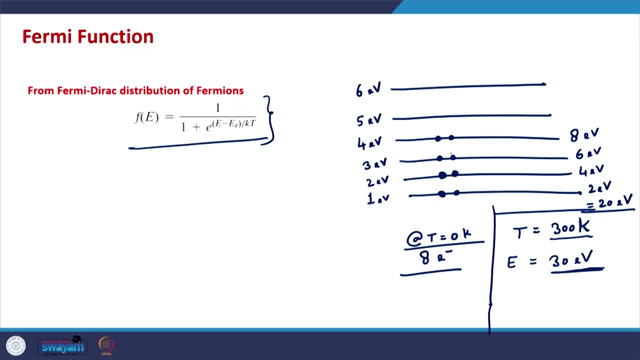 and let us say these 2 electrons, or just for, since we have less number of energy level. let us say we take the energy to be 20. So at t equal to 0 Kelvin, the energy was 20 eV. now let us say the energy is 24 eV. 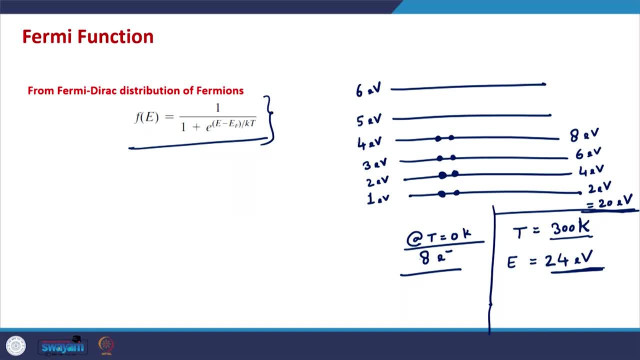 So one of the configurations in this situation will be- please try to guess it- what could be one of the configurations? So one of the configurations would be that this electron, which was earlier sitting here, in this energy level, this might go here, this might go here. 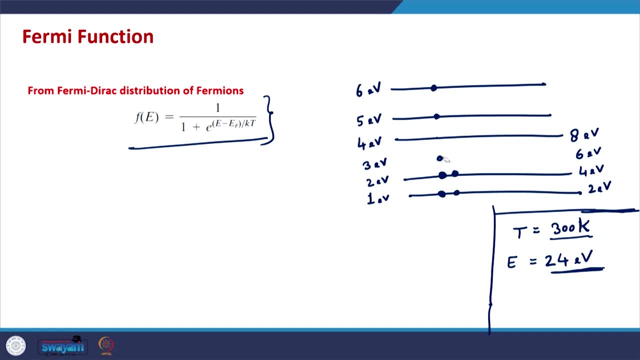 So the energy is now So the energy. so one of the electronic configuration could be this: in this case the energy of the system would be 6 plus 5 plus 4, 15 plus 3, 18 plus 2 plus 2, 22 plus 1 plus 1, 24 eV. So 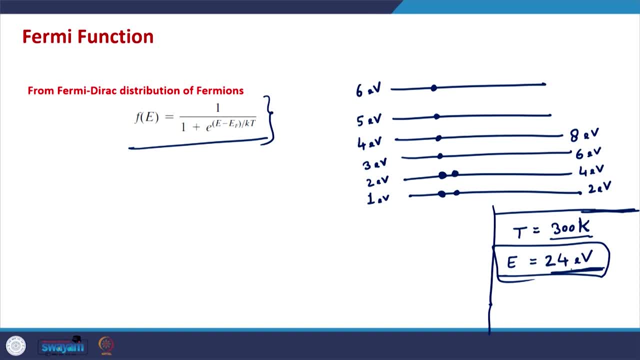 at a certain temperature, if the energy is increased because of the thermal energy, then one of the configurations that the electrons can take is this. Another configuration that the electrons can take is: So it is an interesting exercise to find out how many electronic configurations are possible at 24 eV energy. I would recommend